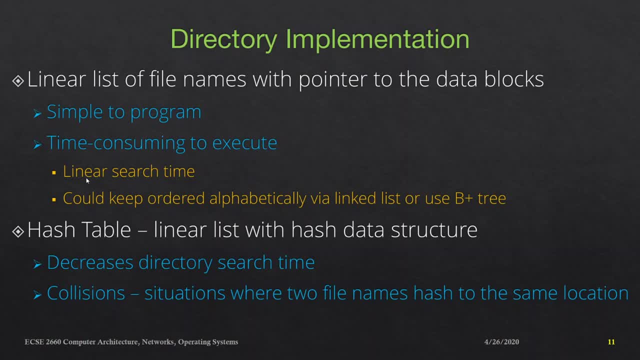 So a regular file name is going to be long because it's a linear search time. So if you're trying to search for the first file in the list, it's going to be very fast, but 50th file in the list is going to take you 50 times longer because it's arranged in the form of a linear list. So we could have 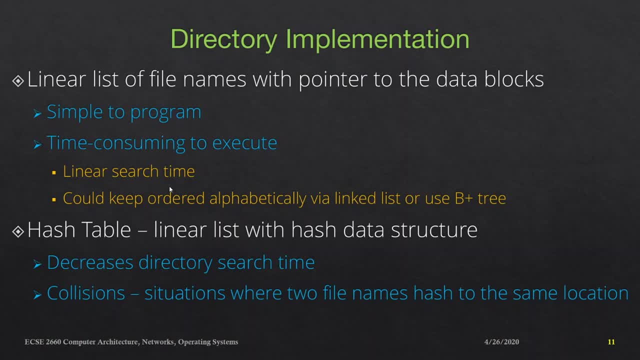 algorithms that search to make our time or latency lower. So we could keep an ordered alphabetically list via linked list or a b plus tree. But the major drawback here is the time it takes to find a file or to verify whether one exists or not. The alternate to that is the hash table. 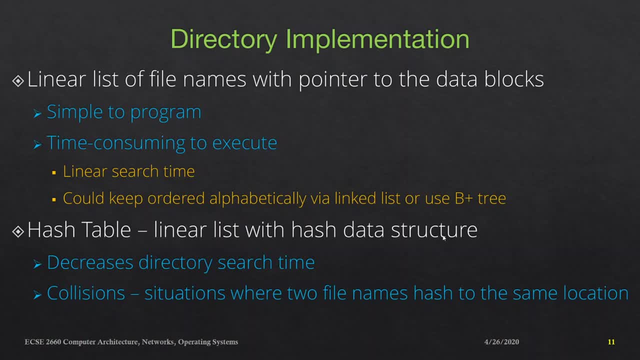 which is a linear list with hash data structure, So a data structure which takes in a file name and gives an output of the file location. So it decreases the data structure, So it decreases the directory search time tremendously. However, collisions is one of the problems. So collisions. 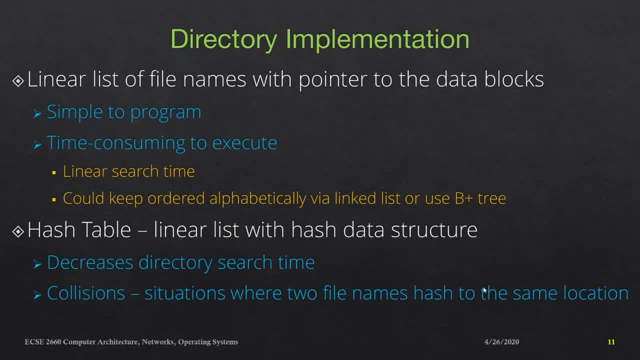 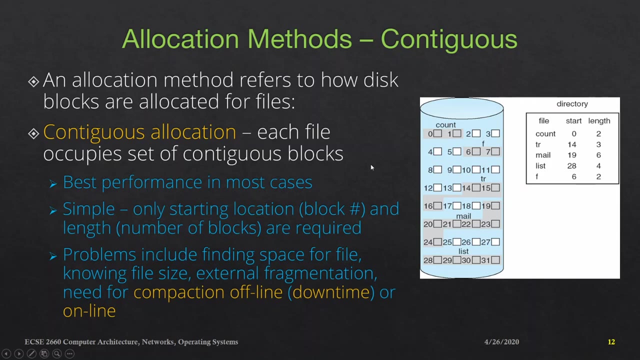 are situations where two file names hash to the same location. So these are two ways how you could run a directory organization. So next we'll take a look at allocation methods. So we are essentially going to go through three different methods of allocating disk space to files We'll talk about. 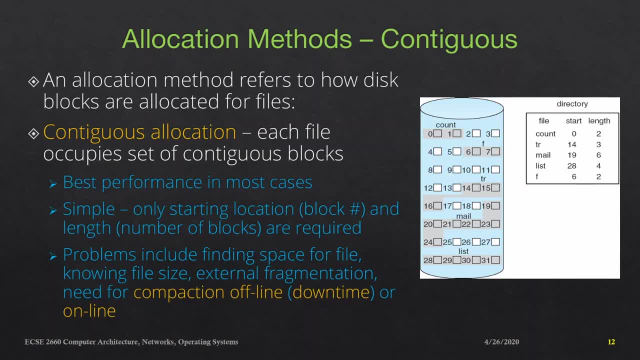 contiguous, Then we'll talk about contiguous, Then we'll talk about contiguous, And then we'll talk about linked list, and then we'll talk about indexed allocation. Allocation method refers to how disk blocks are allocated for files. So in this picture over here we are seeing a cylinder which is 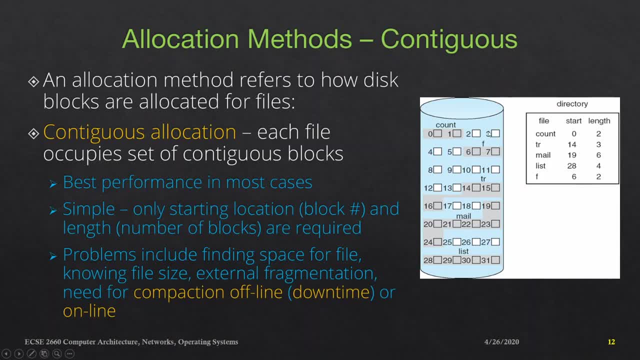 representative of a disk And we are showing different blocks numbered from zero to thirty one. So there are thirty two blocks of thirty two blocks in the hard disk And each block could be used for a file. So, for example, we have a few files here in this particular directory. We have one, two, three. 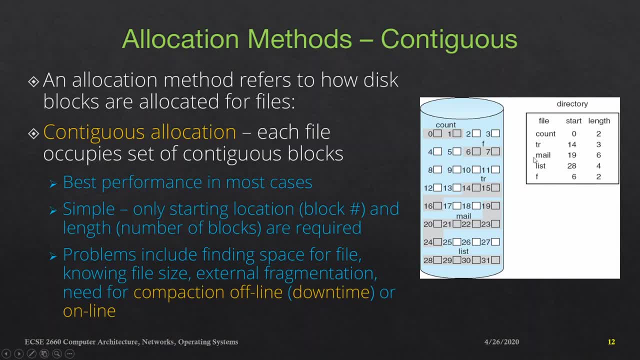 four, five files with file names, count tr, mail list and f And their start block location is given as zero, fourteen and so on, And their lengths are given And in contiguous allocation. this is the case over here. All we need is the start block and the length in terms of number of blocks for each file. 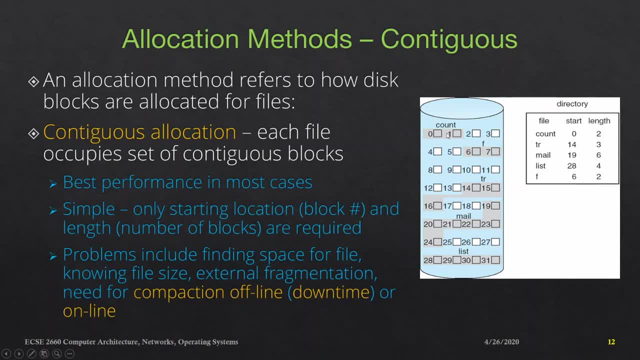 For example, the file count starts at zero and it goes for two blocks, And then the file with file name f starts at six and goes for two blocks, And then you can run down all the all the files here. So it is: each file block occupies a set of contiguous blocks, As you can see here, the all these blocks that are: 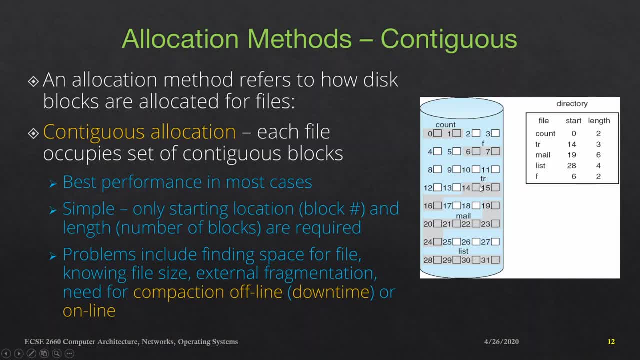 assigned to a particular file name. they are contiguous blocks And there is no break in that allocation. So there are some good things that come out of this, But there are also some negatives. So performance is very fast because reading successive blocks of the same file 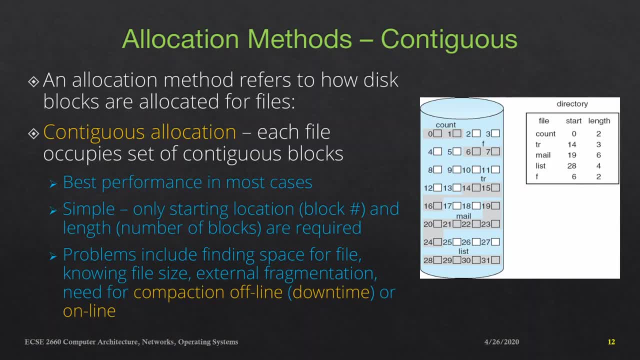 generally requires no movement of the disk heads or at most one small step to the next adjacent cylinder on the hard disk. So that's why it's considered to be best performance in most cases. But problems can arise when files are not in the correct order, For example, if you have a file that 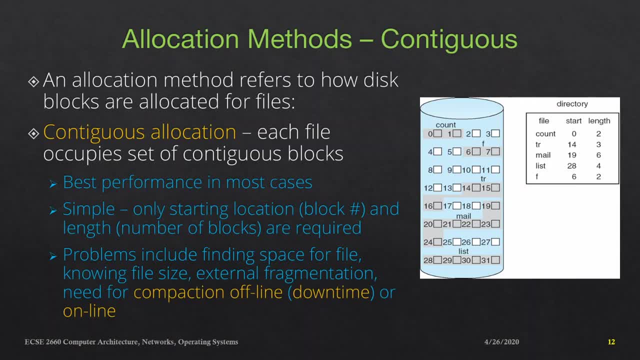 is a little bit larger than the size of the file. you may be asked why the files grow or if the exact size of a file is unknown at creation time. So overestimation of the files final size increases external fragmentation and wastes disk space. So as you can see here there are several blocks that 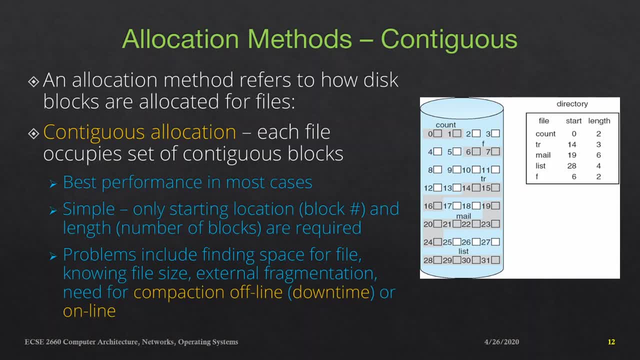 have been fragmented, which is not a desirable thing, And on the other hand, if you have, that may require that a file be moved or a process aborted if the file grows beyond its originally allocated space. If a file grows slowly over a long period of time and the total final space must be allocated initially, then a lot of 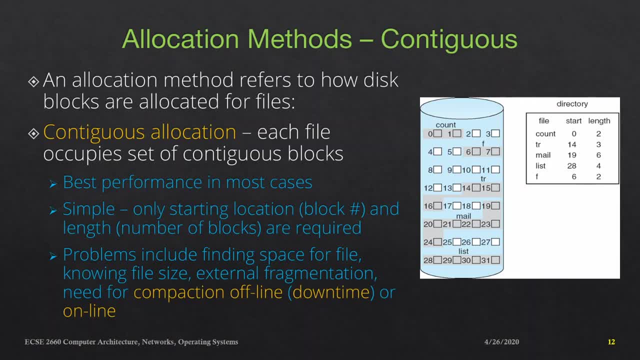 space becomes unusable before the file fills the space, So that is not a very good utilization of the memory. Another drawback here is the need for compaction, either offline or online. Compaction is a process of making free blocks into contiguous blocks so that we can fit in bigger files in those spaces. 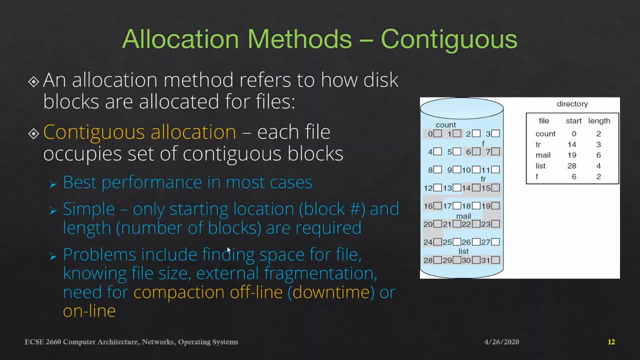 So we will need compaction when we do contiguous allocation. Another good thing about contiguous allocation is, even if there is a certain virus that corrupts a particular block, the remaining blocks will be still intact, so it's not like we are going to lose the complete file, although even though there 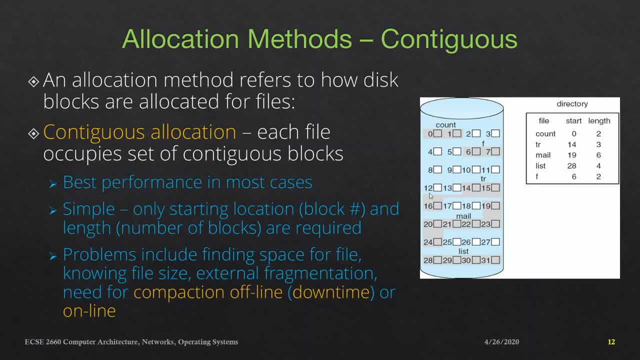 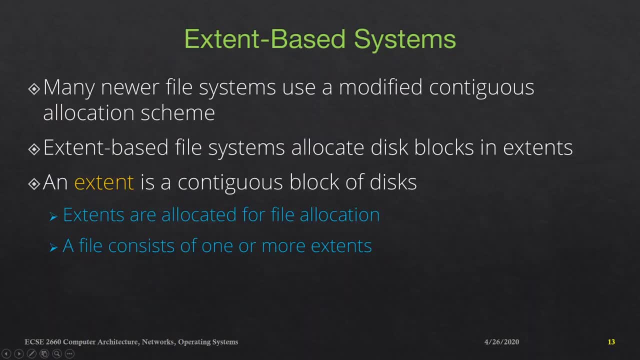 are some blocks. they might that might be corrupted, so we'll still have some data of the file that is preserved. extent based files are an alternate to contiguous allocation, so a variation is to allocate file space in large contiguous chunks. they are called extents. when a file outgrows, 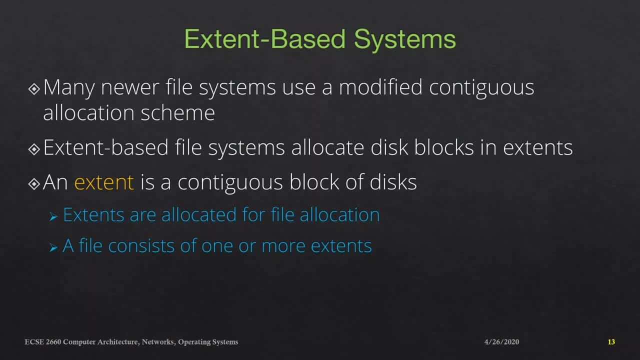 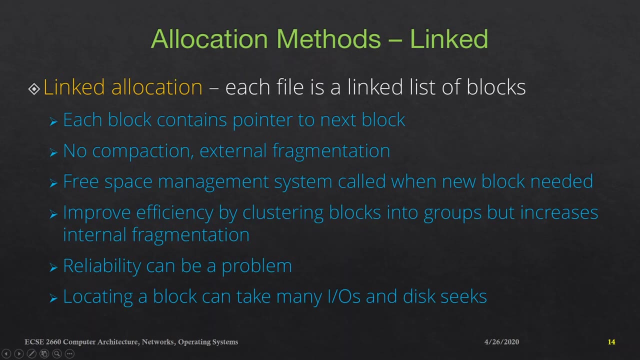 its original extent, then an additional one is allocated. the high performance file system veritas, which is supported by linux, uses you extends to optimize performance. so next let us take a look at linked allocation method. disk files can be stored as link list, with the expense of the storage space consumed by each link in the link list, each block. 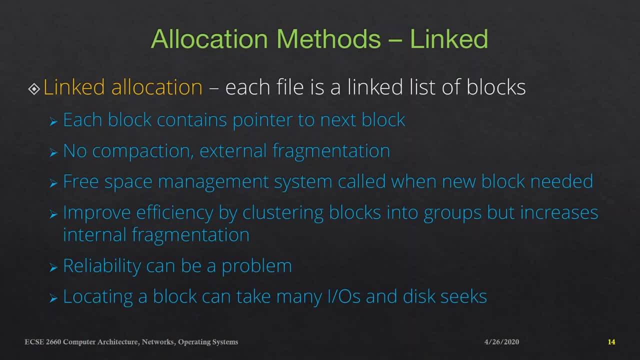 contains data of the file and pointer to the next block. linked allocation invents a link to the next block and points it to the next block, involves no external fragmentation, does not require pre-known file sizes and allows files to grow dynamically at any time. unfortunately, linked allocation is only efficient for sequential access. 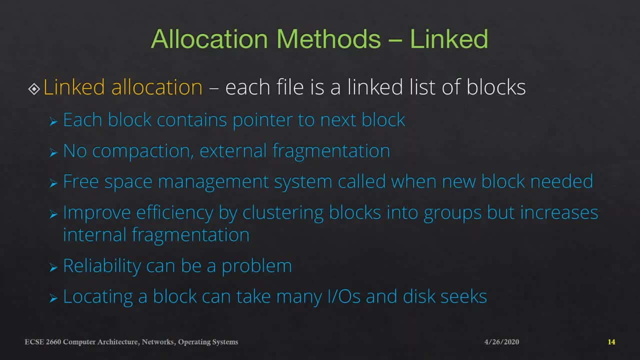 files, as random access requires starting at the beginning of the list for each new location access. allocating clusters of blocks reduces the space wasted by pointers at the cost of internal fragmentation. another big problem with linked allocation is reliability of a if a pointer is lost or damaged. a doubly linked list provide some protection at the cost of additional overhead and wasted space. 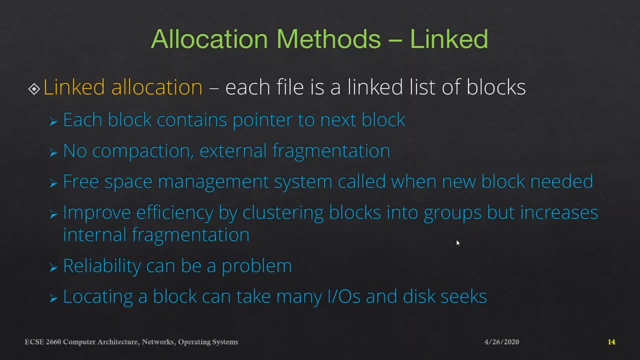 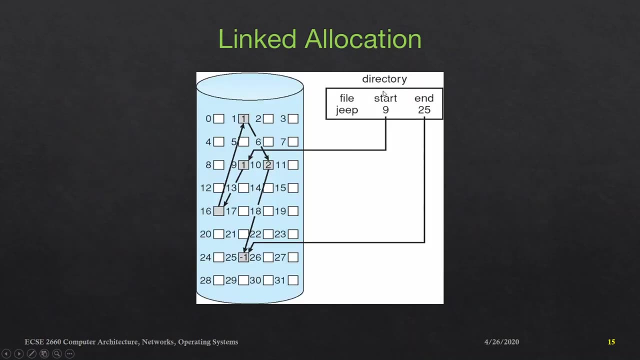 so those were some of the advantages and disadvantages of a linked allocation. let's take a look at how it works over here. so there is one file with the file name jeep in the directory that is, and all the information that we need is the starting block and the ending. 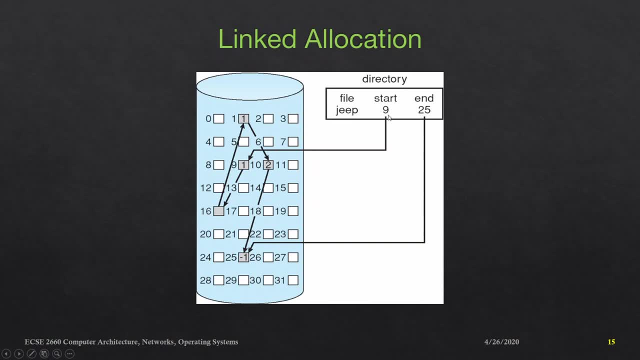 block and if we start accessing the, the first block 9, we are going to look at block number 9, which contains part of the data of that file, jeep, but it also contains the pointer to the next block. so in this case it is going to go from block 9 to 13, to 16, to 1 to 6, to block 10, to block 18, to 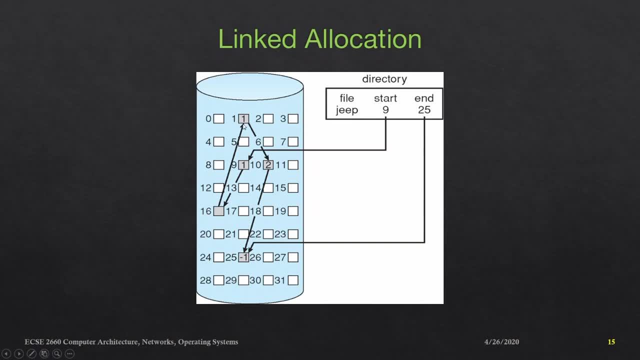 block 25, which is the ending block. so that particular link is the linked allocation. so all those blocks have two things: one is part of the file and the other is the pointer to the next block. one problem that could happen over here is if the point, if the link breaks, then we lose the good portion of the file. so we we can. 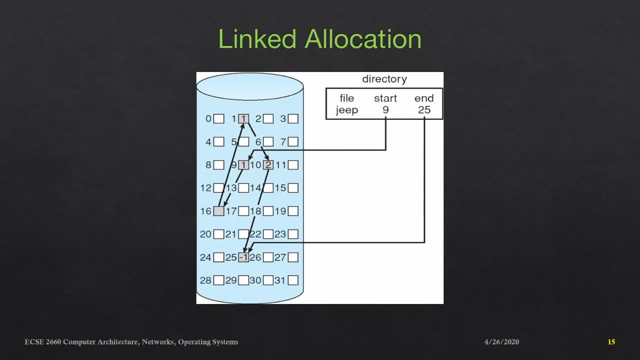 go for the doubly linked approach that we used for unix file system inode, in which we had single pointers, double doubly linked pointers and triple linked pointers. so we could use that approach to kind of overcome that problem. but in this case all we need is the start and end block number and everything else is linked. 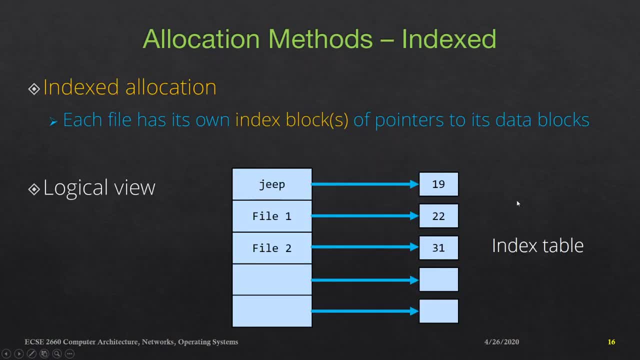 now let's talk about indexed allocation. so in indexed allocation we have each file which has its own index blocks of pointers to its data blocks. so, as we can see over here, there are several files on the left: jeep, file 1, file 2 and so on, and we can see that there are several files. 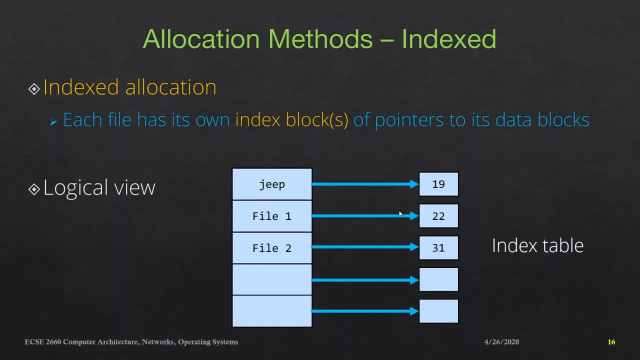 on the right, jeep file 0, and so on, and we can see that there are several files on the left, jeep file 3, and so one 0 and in this particular index tools that we learned summarized, the first class inра is said: oh, number of the index block we take. 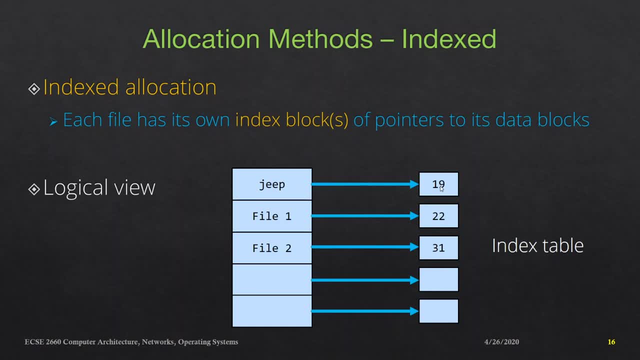 0. there is a number 0, dot. itlet not proceed. 0 dot, dot, dot, dot, delta dot, or something like that. and at its index block, what a db themselves they will be. obưởng ore in r to all of its data blocks. now let's take a look at the a- g example of its. so, essentially, what we are doing is we are combining. 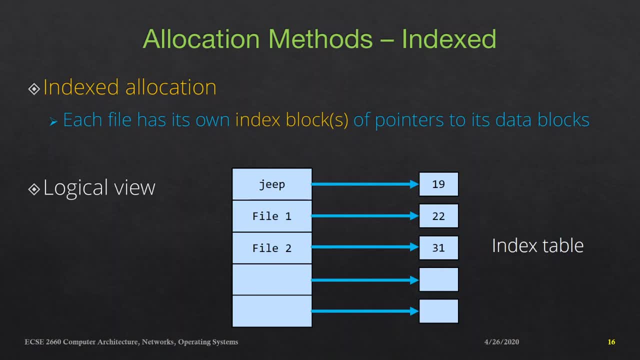 all of the index loot by just parts of our index file, so by stuffback g我们 all of our in dc's block are pitch each file into the common block les place he lecture teachers common block called the index block. Inde vivac random becomes normal. correlate: all the index, all index functions. expect to can make Hebrew Exam. 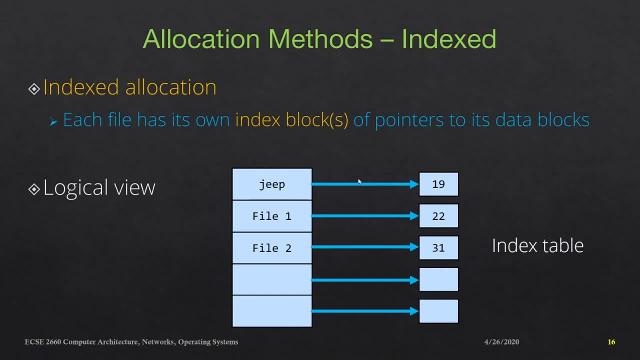 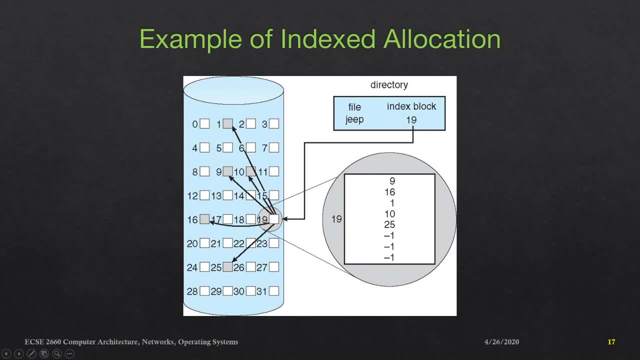 block for that particular file, as opposed to spreading them all over the disk. So in this picture we can see how the file jeep, which has the index block 19, and if we look- go and look into index sorry, block 19, we can take a look at the. 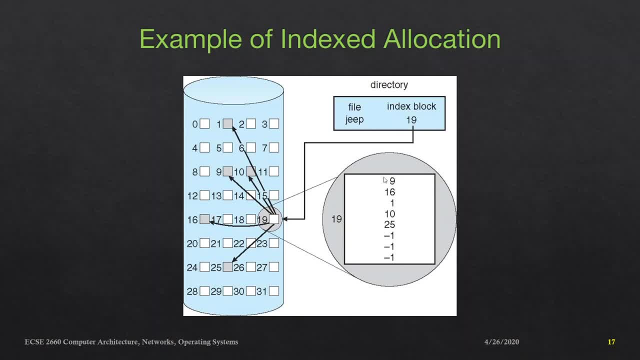 pointers to all the data blocks. so this particular file, jeep, is present at blocks 9, 16 and so on, up to 25 and 3 of the blocks are not being used because in this case we have 8 blocks per index file, per index block. So clearly some 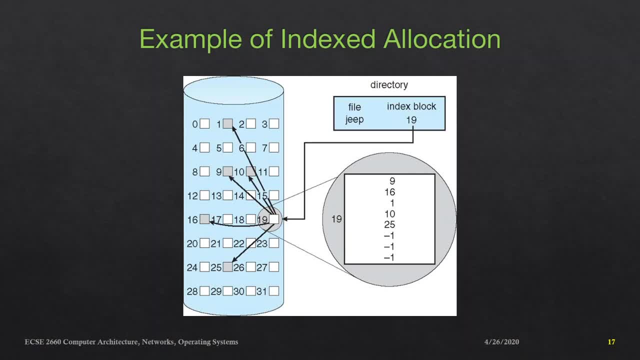 disk space is wasted because an entire index block must be allocated to each file, regardless of how many data blocks the file contains. So this actually leads us to questions of how big the index block should be and how it should be implemented. So let's take a. 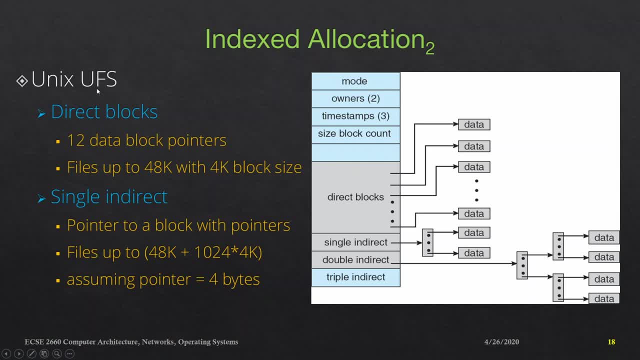 look at that with how Unix does it in its Unix file system. So the inode, which is essentially carrying the metadata information for each file, has direct blocks, single indirect blocks, double indirect blocks and triple indirect blocks and there's a. there's a big advantage of doing this because we can. 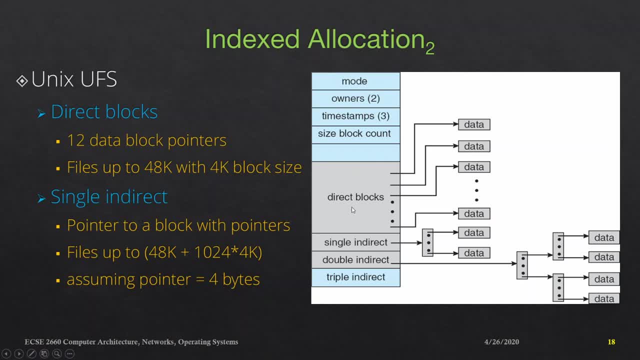 access small files very, very quickly, and if we have a very, very large file, then it's going to take us some time, but it's it's. it's going to be an increment of of time, very. it's a slow increment of time, but but by doing this we can have a very 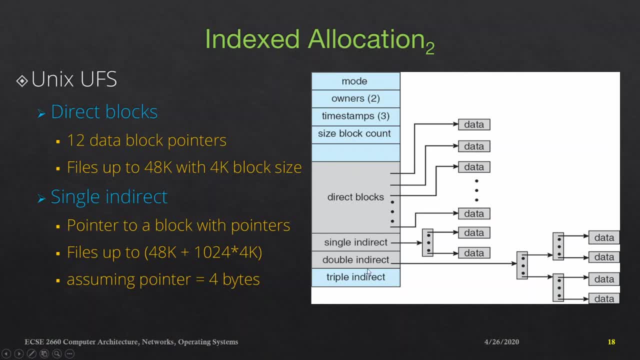 very large amount of file that we can have on the hard disk. So let's see how to how to understand this inode structure for Unix file system. So there are direct blocks, as you can see here, and direct blocks essentially have 12 or so data block pointers. so essentially, if 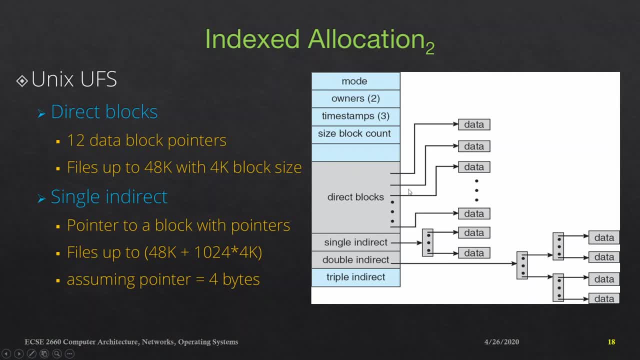 you have 12 pointers to data block and if the file is small enough to fit those twelve data blocks, then we are done and all you have to do is take a look at those pointers and access those twelve blocks. So files up to a size of 48 K if 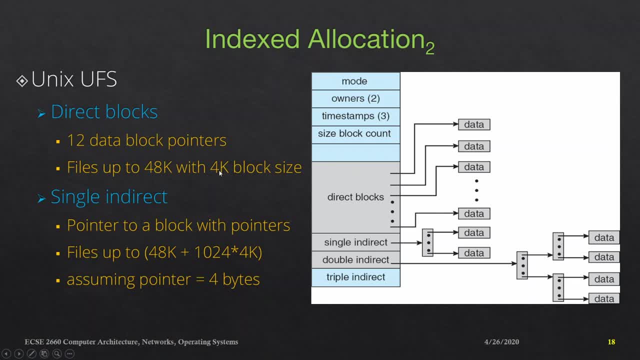 you assume a kilobyte block size, we can fit using just the direct blocks which are going to be cached so they can be accessed very, very quickly. now if the file size is a little bit larger, then we are going to use direct blocks as well as the single indirect. so a single indirect is essentially 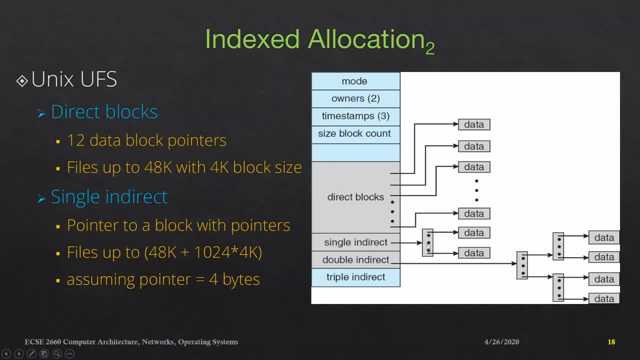 there is a. there is a pointer to a block which contains pointers to where the data is and in this case files up to you know. the sum of these two sizes can be used using direct plus single indirect, so the 48k number is coming from direct blocks, which was already there.